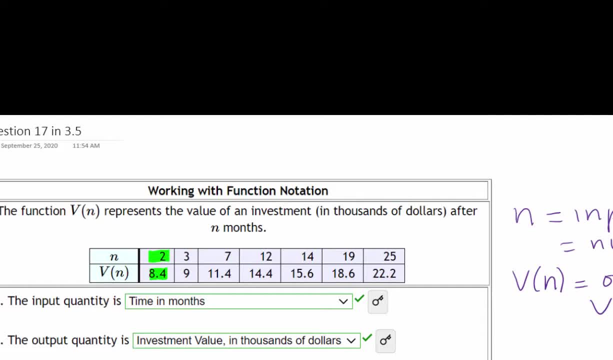 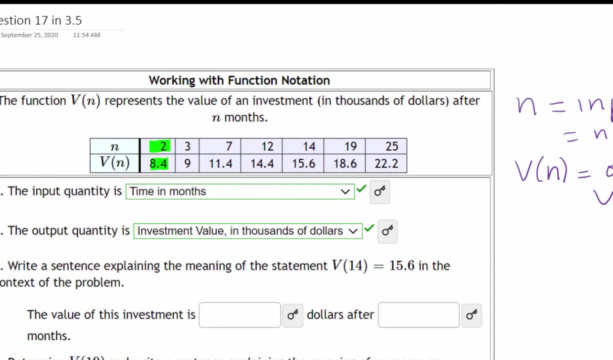 We talked about that as the number of months of the investment and the output quantity or the output variable is the investment value in thousands of dollars. So we know that Now it says here: write a sentence explaining the meaning of the statement. V of 14 equals 15.6. in the context of the problem, 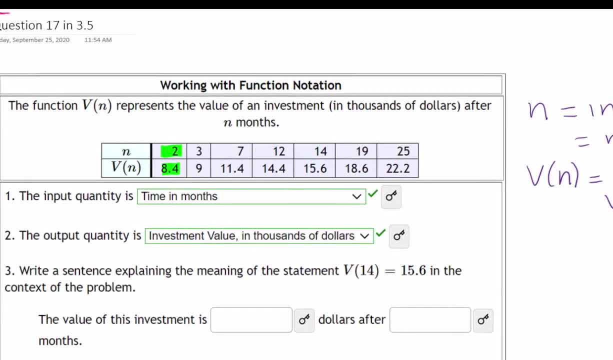 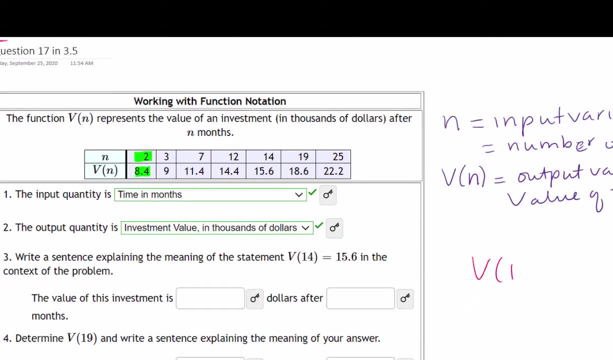 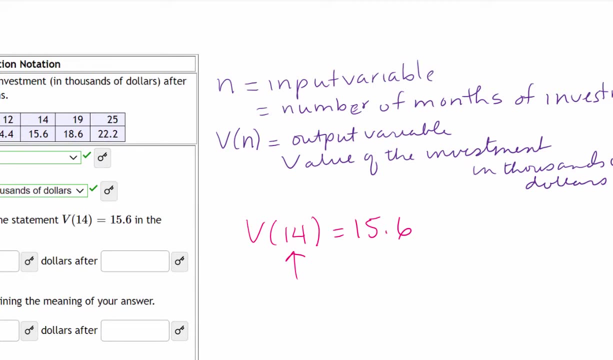 So, once again, what does that represent? Well, remember that in function notation, and that's right over here, if I have V of 14 equals 15.6,. this number, that's in this parenthesis, that's your input coordinate. okay. 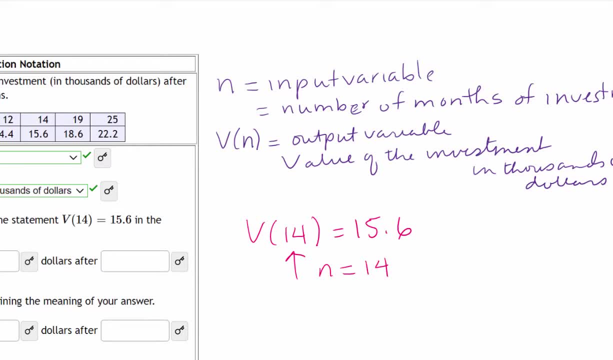 So that means n is 14, and then the 15.6 is our output. So that means that 14 months After we have this investment, the investment is worth. so, remember, the output is the value of the investment. so this 15.6 times 1,000, because, remember, it's in thousands of dollars- so $15,600 is the value of the investment. 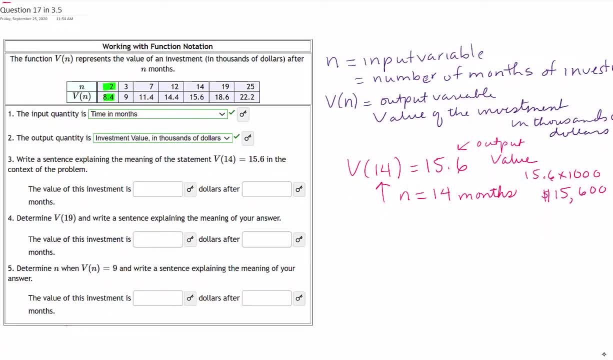 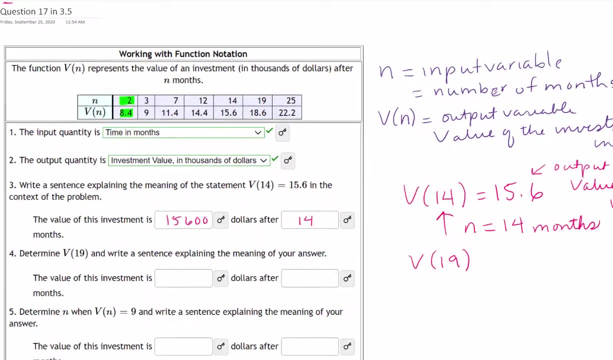 So again, the value of the investment is $15,600 after 14 months, And that's what the notation represents. Okay, so V of 19,, V of 19,. so let's go look up here at the table. 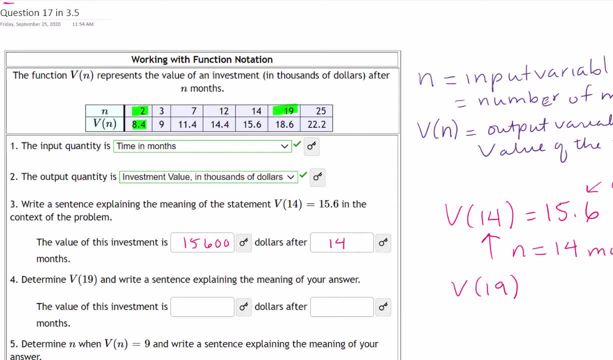 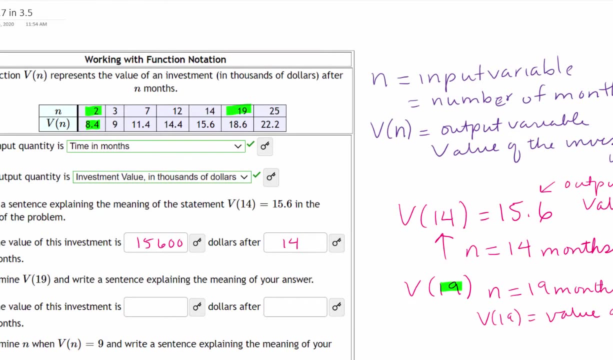 Okay, so here's 19, because, remember this, 19 is your input, so that means the number of months. so 19 months, And you're being asked to find V of 19 is the value of the investment after 19 months. 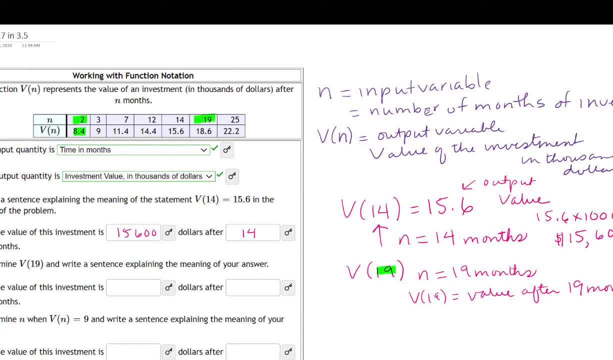 Okay, so that's what the notation- So let's look at the table- tells us, right? The table says: when n is 19, V of n is 18.6, and remember you're multiplying that by 1,000, because those are dollars. 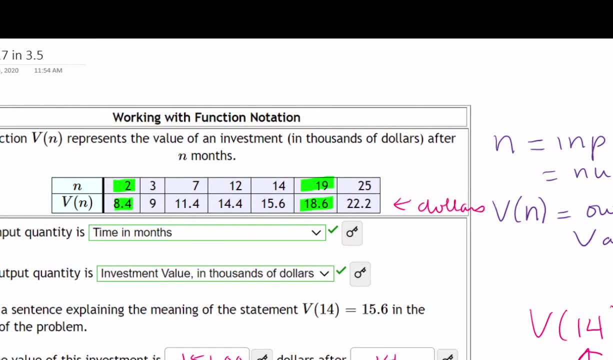 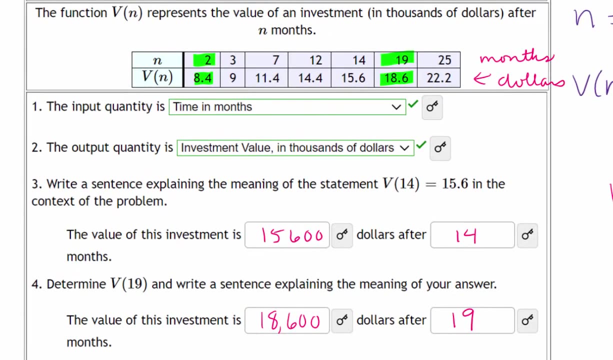 So we have here- let's put this here- dollars months. okay, Just label our table there, that might help. So the value of the investment is $18,600 after 19.6.. Okay, so now let's look at number five.